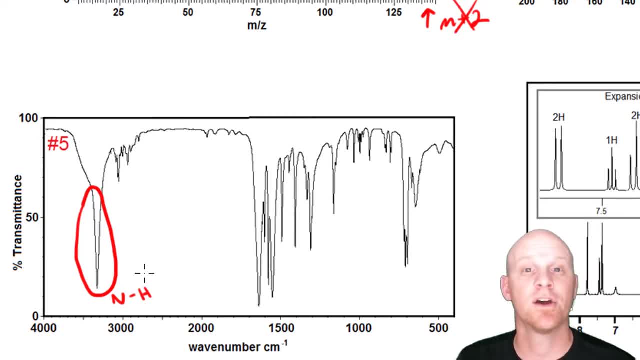 it's convenient: One peak, one hydrogen attached to your nitrogen, two peaks, two hydrogens attached to your nitrogen, And so in this case it's just one peak, So there's just one hydrogen attached to our nitrogen. If we also show we have peaks just left of 3,000 and peaks just to the right, 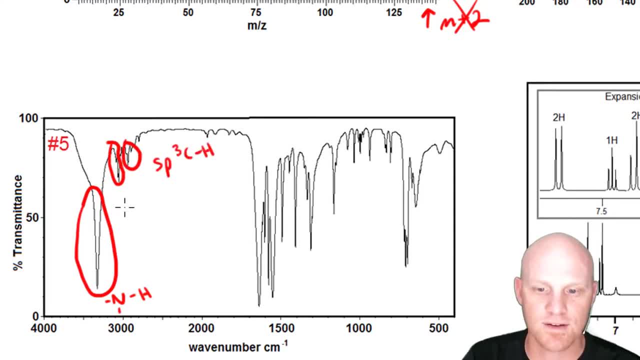 of 3,000, and again that's your sp3ch bonds just to the right and sp2ch bonds just to the left of 3,000.. And then working our way down here and again. usually we'll kind of 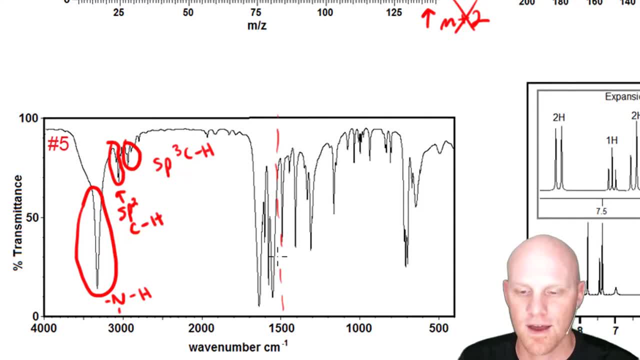 take 1,500 and ignore everything past that, And we've got a bunch of peaks immediately to the left of 1,500.. So the 1,500 to 1,600 range, that's your aromatic carbon-carbon peaks. So, and this is- 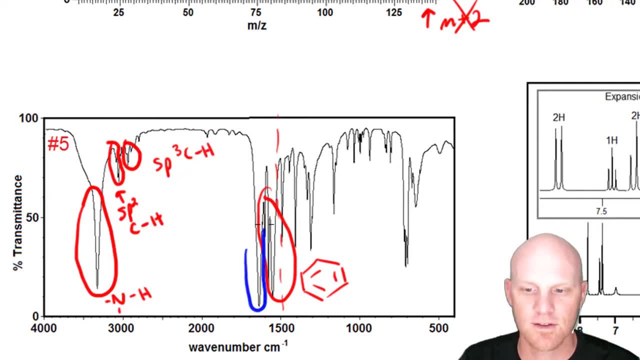 going to be tricky and you might not have caught it, but technically this signal right here is a carbon-oxygen double bond. Now, normally we think those show up at 1,700.. This one actually looks like it's closer to 1,600 than 1,700.. So somewhere between 1,600 and 1,650.. So it's. 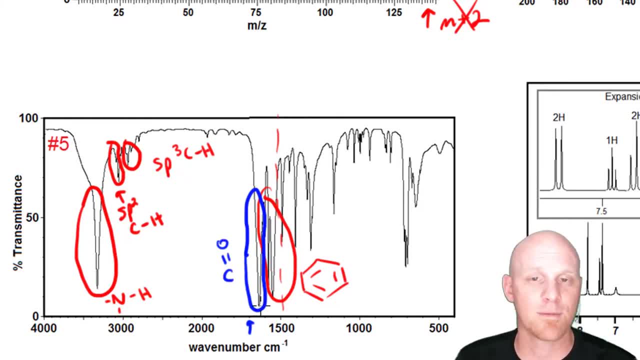 definitely experiencing some conjugation. We'll find out. it's an amide in a little bit, but we'll find out it's even more conjugated than that. But in this case, even if we didn't realize, we had a carbon-oxygen double bond from the IR. the carbon-13 NMR would make it very obvious. Let's 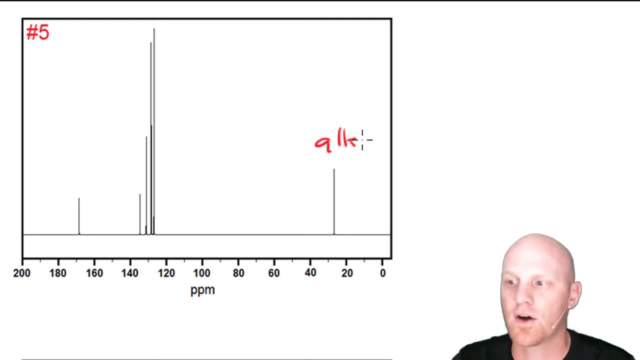 take a look. So here we've got a signal down here in the alkane region, So, and then we've got four signals over here in the 110 to 160 aromatic regions. So we've got a benzene ring And then we've got a carbon double bonded oxygen- The only thing that shows up downfield of 160.. 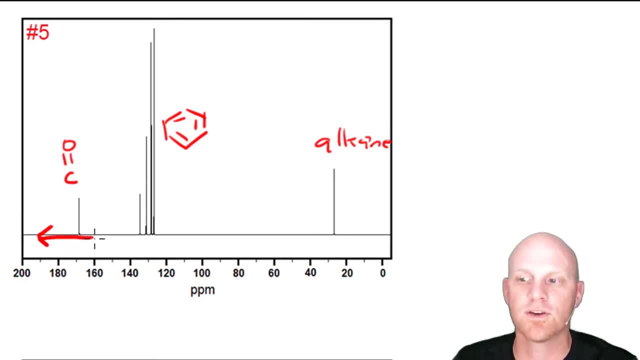 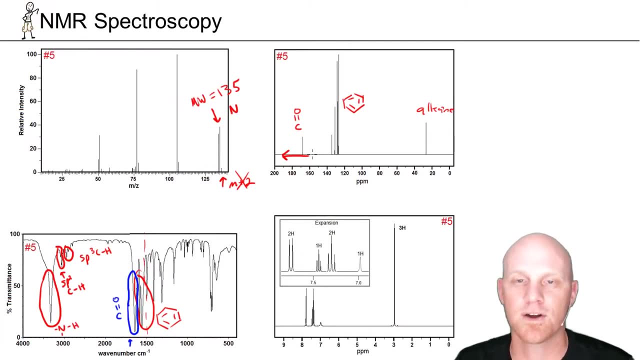 So again, if we didn't realize we had a carbonyl before with the IR, we definitely couldn't miss it here in our carbon-13 NMR And yet again take what we know now and finally spend the most amount of time in our HNMR spectrum. So now let's spend some time looking at the 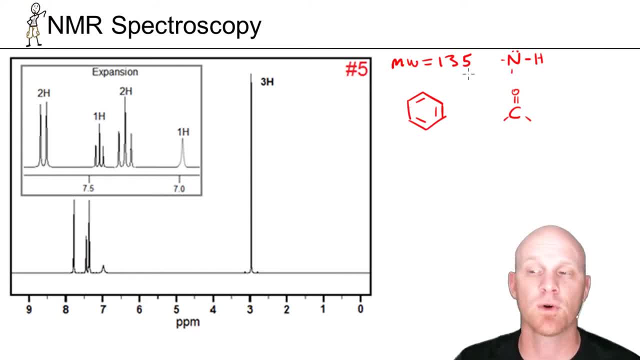 HNMR And I've summarized our findings from the other three spectra. Our molecular weight is 135.. We have a nitrogen and it's bonded to one, hydrogen. We have a benzene ring carbonyl. If we move on here, let's spend some time. We've got a number of signals. We've got. 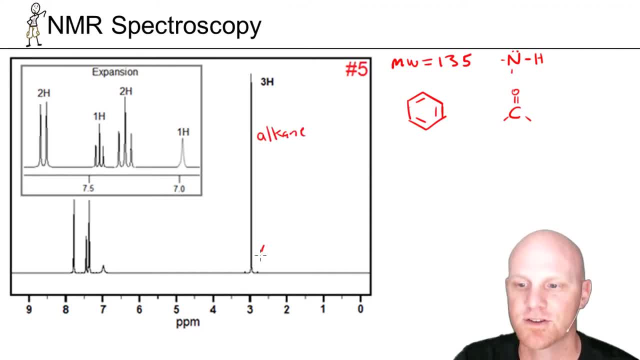 one down here in the alkane region And it looks like it's showing up just shy of three. Maybe it's right next to something electronegative, Maybe it's not, But it's definitely in the alkane region. And then we've got all these signals down here that look like they're in the aromatic region. 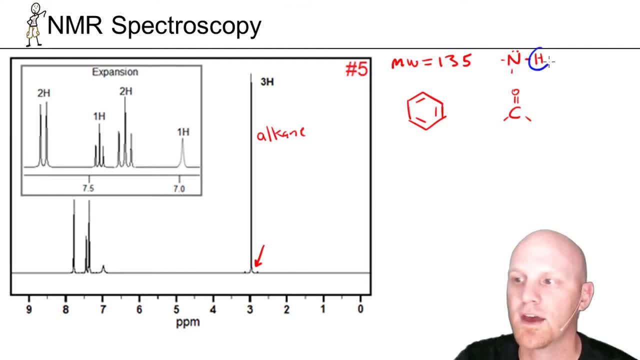 But in this case I would recommend you find where this H attached to the nitrogen is actually showing up. NHs and OHs can show up just about anywhere, depending on what molecule they're in, depending on what solvent you're using. So I highly recommend you find them, And NHs and OHs are often broader than most other peaks. 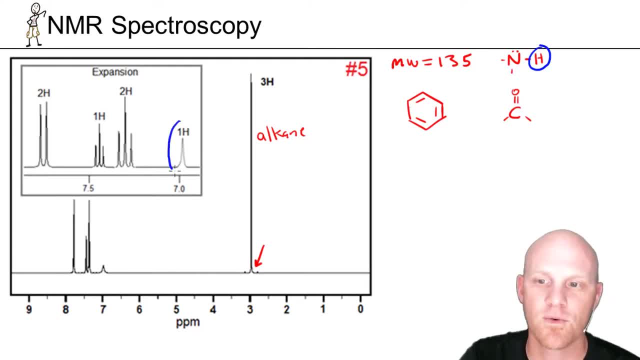 and they're typically broad singlets. And in that case that's this guy right here showing up at seven. So have we not identified him from the get-go? We might have thought he was another aromatic hydrogen, But in this case he's the NH. He's that broad singlet. So getting him out of the 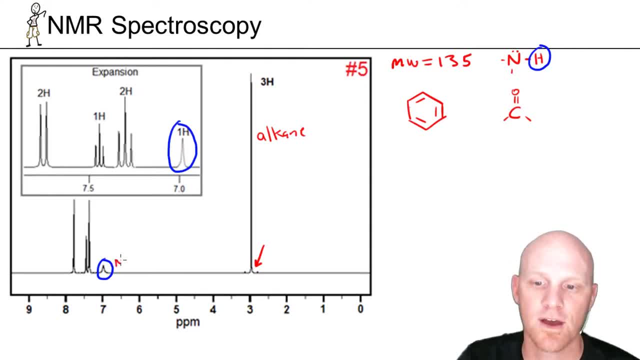 way early is going to help us big time. So that's our NH again, And then these other signals, these are the aromatic ones, So it's hard to distinguish, and that's why you're given an expansion here, a blow-up of that region. 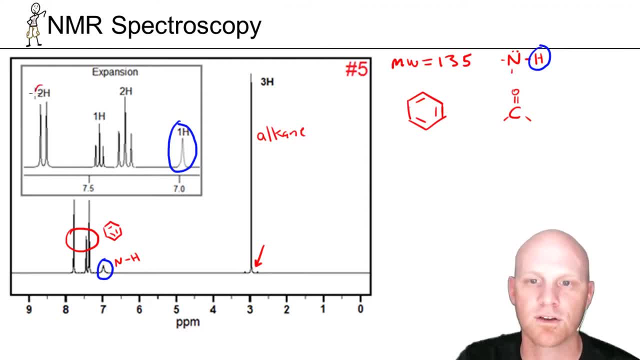 And the important thing is not looking at all these signals. The important thing here is first and foremost going to be looking at your integration. So in your integration here, 2 to 1 to 2 ratio, that's a total of five hydrogens And that's super nice. This is your other common aromatic. 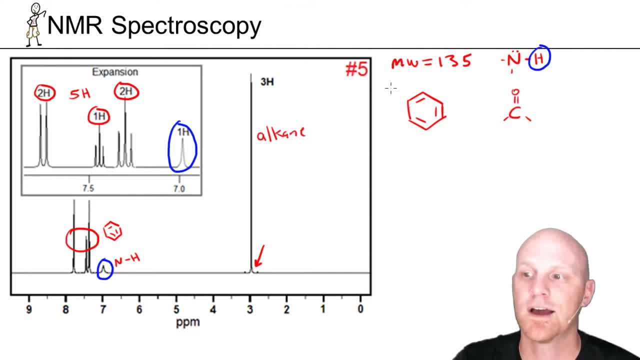 pattern that routinely shows up in an undergraduate class here, And that's a monosubstituted benzene ring here. So we have one substituent. The other five positions are all going to be hydrogen And that's going to be your hydrogens in all likelihood. And whether I analyze all the singlets and 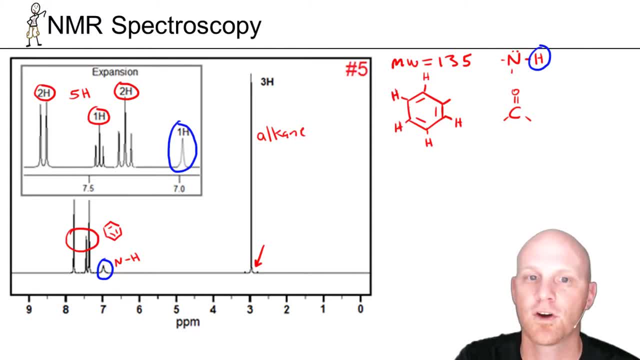 doublets and triplets. it's not the most crucial thing in the world, But if you look at this thing, there is going to be symmetry here. It's going to reduce the number of signals, It's going to make these two Hs equivalent And in this case they're only going to have the one neighbor next to them. 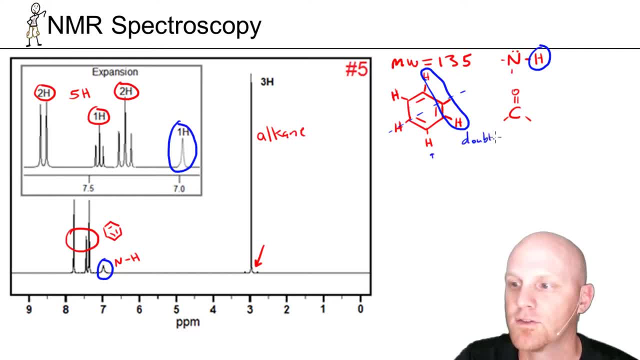 here And, as a result, show up as a doublet. So then you've got this guy down here And he's got these two neighbors here again. So he's going to be a double. So he's going to be a double And I'm going to. 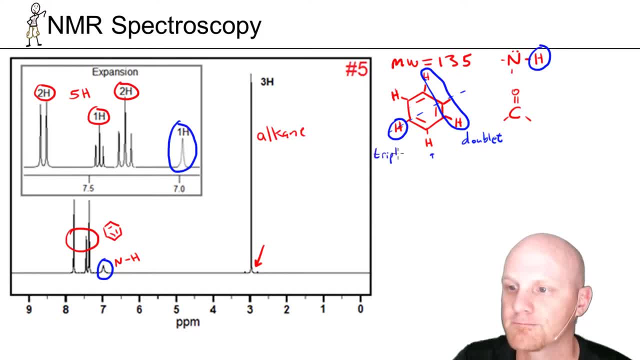 It's going to be a double, So I'm going to be a double, So he's going to be a double And I'm going to. you would show up with two neighbors as a triplet, And then you have these two hydrons being equivalent. 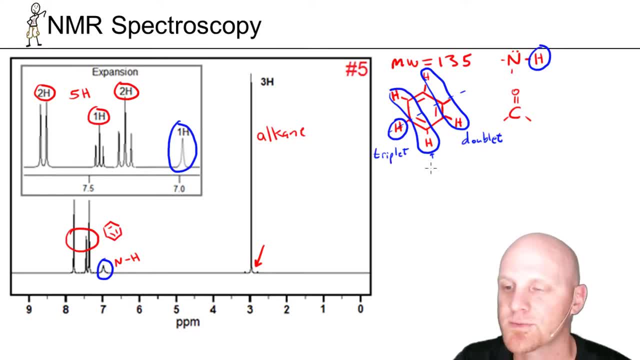 So these guys got a neighbor on either side and they're non-equivalent neighbors. So technically there's some complex splitting on here. But oftentimes the complex splitting on here ends up looking a whole lot like a triplet, even though it's technically a doublet of doublets. 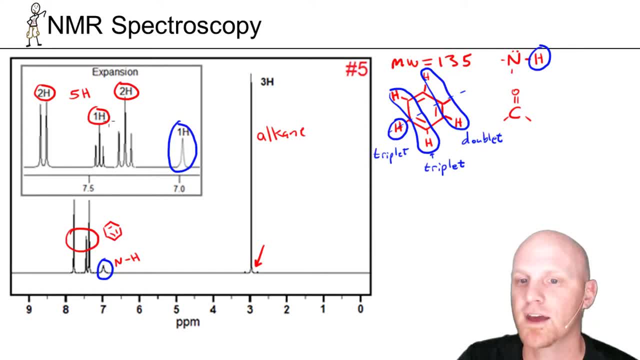 But in this case that's exactly the pattern. I see a 2H doublet, a 1H triplet and a 2H- something that looks like a triplet. that's technically a doublet of doublets, But we'll talk more about complex splitting later. 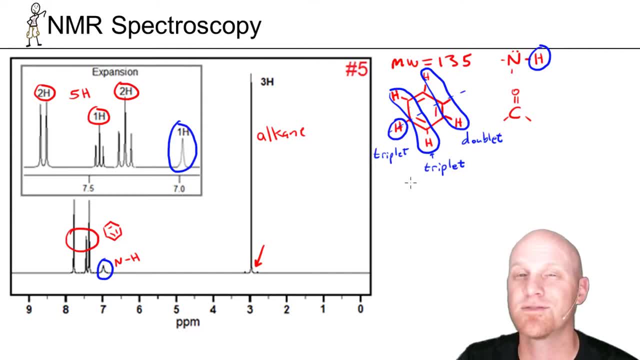 But that exactly matches our pattern. But whether we realized it matched or not, once you see 5Hs in the aromatic region. so you almost definitely have a monosubsidated benzene ring, if you don't have more than one benzene ring anyways. 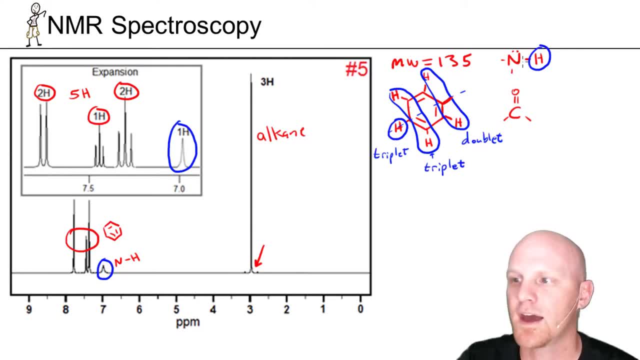 And so in this case, that's what we have And that's a piece of our puzzle. So we've got the nitrogen here, We've got this carbon here, We've got the benzene ring, And then we've got these 3Hs in the alkene region, which again 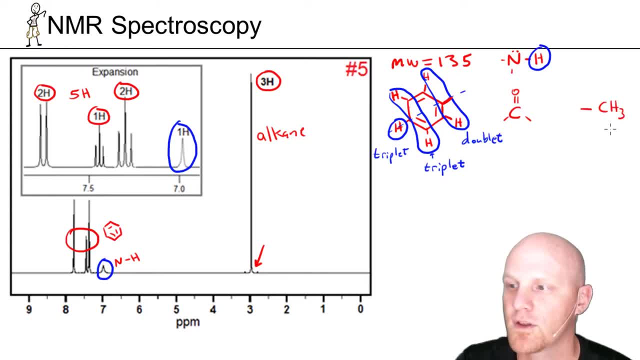 I like, And that's going to be a methyl group. So in this case that's about all we know. If we kind of take a look here, our methyl group only has one bond left to make. It can't go in the middle. 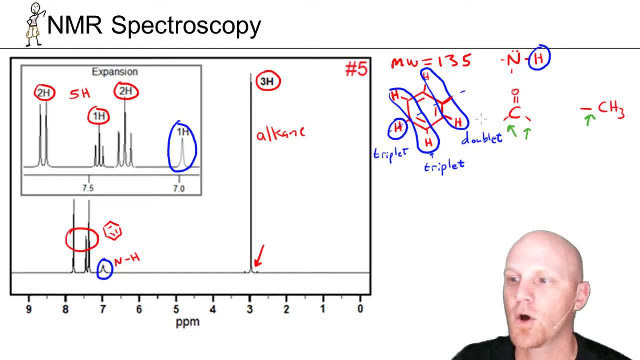 It goes on the end of the chain. Our carbonyl has two bonds to make. It can go in the middle. Our benzene ring only has one bond to make. It can't go in the middle. It has to go at the end of the chain. 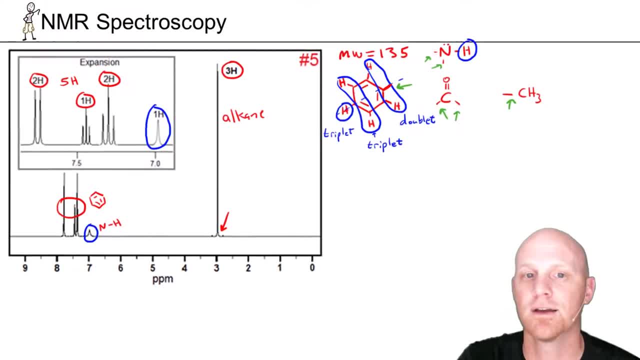 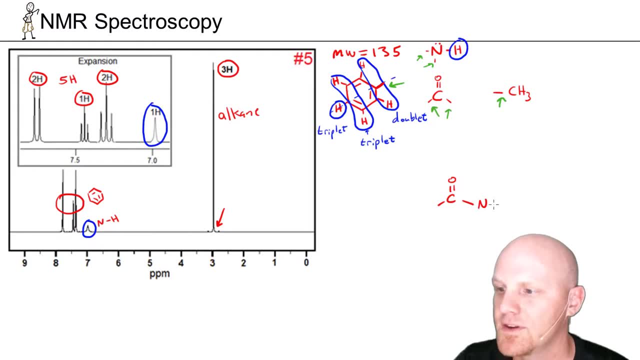 And then our nitrogen has two bonds to make, So it can also go in the middle of the chain. So our two fragments that can go in the middle of the chain here are the carbonyl and the nitrogen, So we'll attach them to each other. 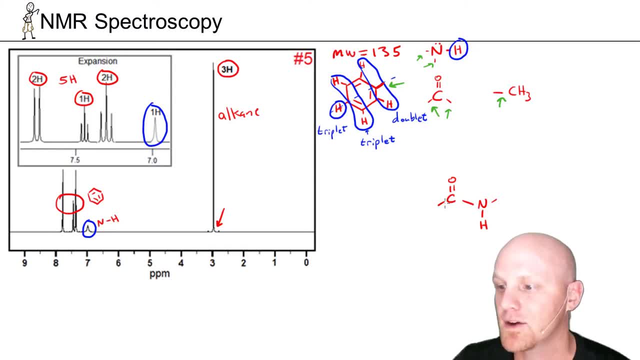 And then, in this case, the nitrogen also had the hydrogen, And from here we have two options: I can attach the benzene on the left and the methyl on the right, or exactly the opposite, And so we're going to end up with two possibilities here. 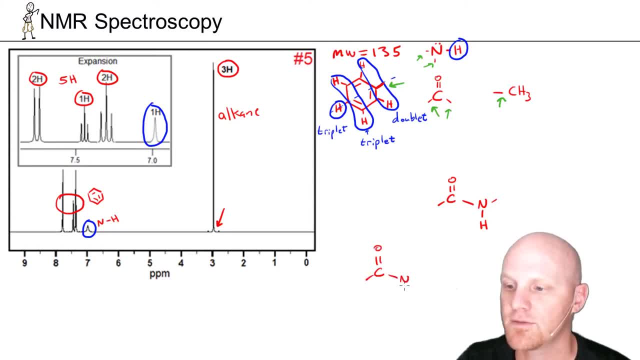 And let's draw both possibilities and see if we can tell the difference. So this is a fairly complicated example here. In this case, I'll start by putting the benzene here and the methyl group here And this one. I'll put the methyl on the left. 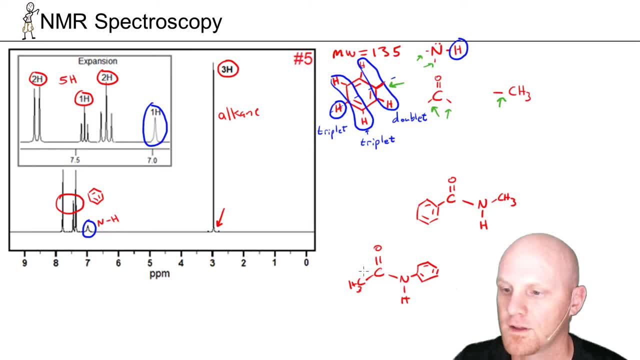 and the benzene on the right. Let's see if we can tell the difference here. So if we look, it turns out this is actually the correct structure. It's going to be a little bit subtle, but there's going to be a couple things that could clue us in. 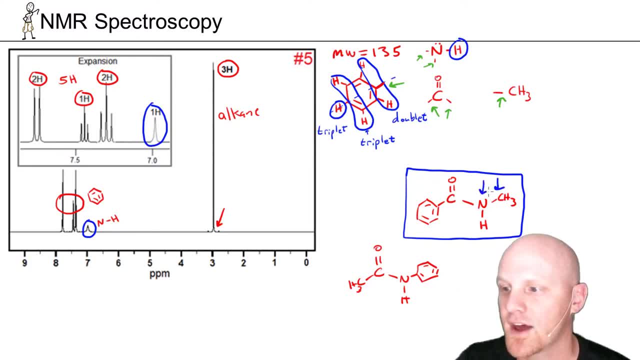 One is the methyl group here, And the methyl group is next to the nitrate. It's bonded to the nitrogen, which should get it down in the three or lower range, And unfortunately this carbon is just barely below three. But maybe he's bonded to the nitrate.